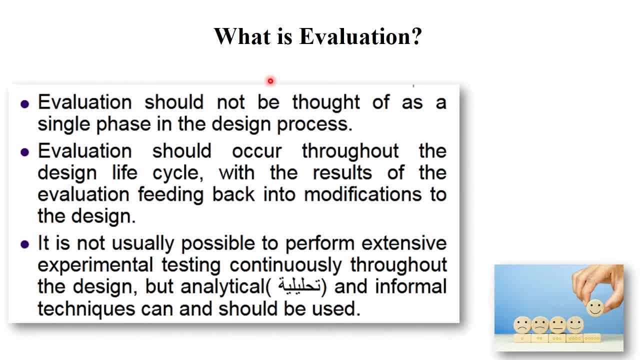 Next. So what is evaluation? Evaluation simply means assessment to check the particular system or the particular model that will be work properly or not. So evaluation should not be thought as a single phase is in design process. Evaluation should occur throughout design lifecycle. 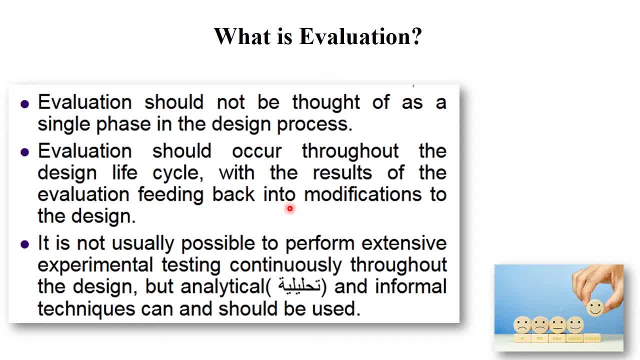 With the result of the evaluation feeding back into modification to the design. So evaluation should occur each and every lifecycle stage, that is, in planning, in requirement gathering, in design phase, implementation phase, testing phase, etc. So it is not usually possible to perform extensive experimental testing continuously throughout the design. 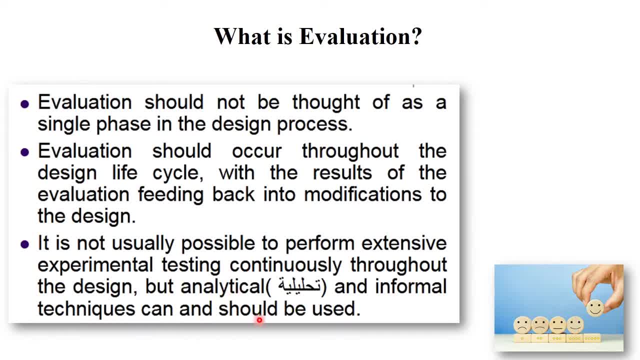 But analytical and informal techniques can and should be used. So evaluation should occur throughout the design. So each and every phase required evaluation- assessment that your software will be exactly matched with the user's requirements or not. So this concept is called as evaluation. 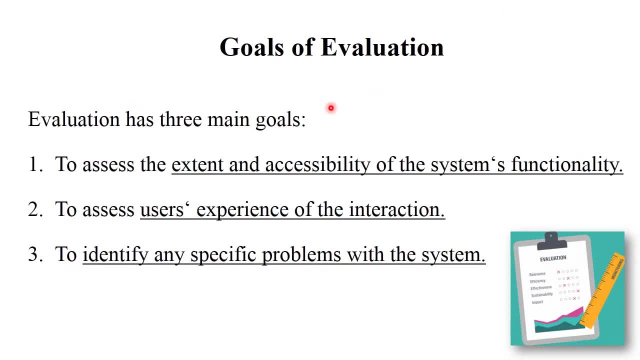 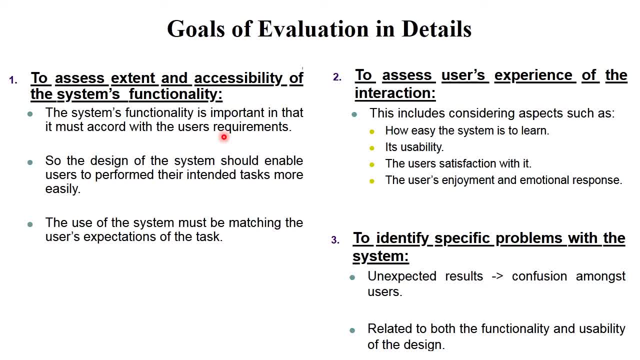 with the user's requirement means your system match with the user's requirement, So the design of the system should enable users perform their intended task more easily. If your design is correct, then implementation will be work properly, right. So the use of system must be matching the 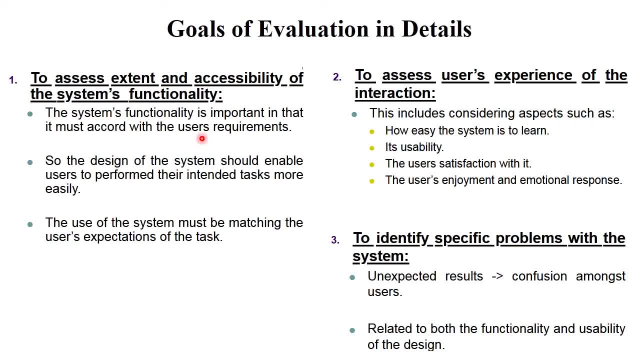 user's expectation of the task clear. So this is your first goal. Next, to assess the user's experience of the interaction. This includes considering aspects such as how easy the system- easy to learn, So usability is one of the most important point while implementing or developing. 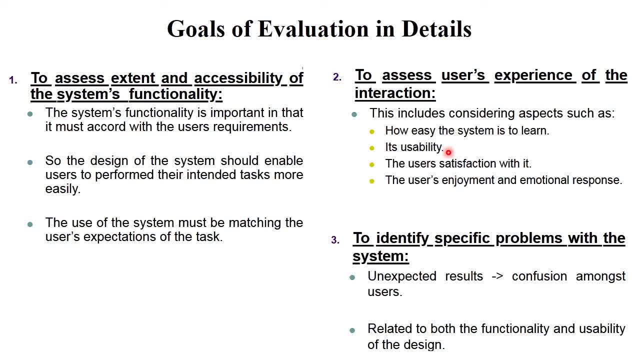 a particular product that will be easy to use and easy to learn. The user's satisfaction is mandatory and the user's enjoyment and emotional response is also a mandatory. This is your second goal. okay, Next, to identify a specific problem with the system. Suppose unexpected result will be generated. so there is a confusion amongst the users, right? 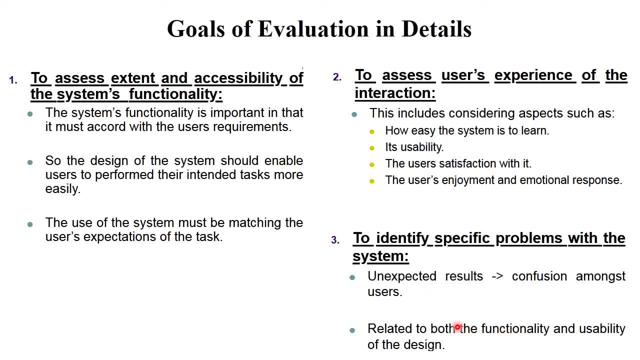 So, related to the, both the functionality and usability of design, you should develop a particular software, For example. if something went wrong, then there will be a particular options available. that is help, etc. right, So this is the concept or goal of evaluation in detail. Next evaluation: 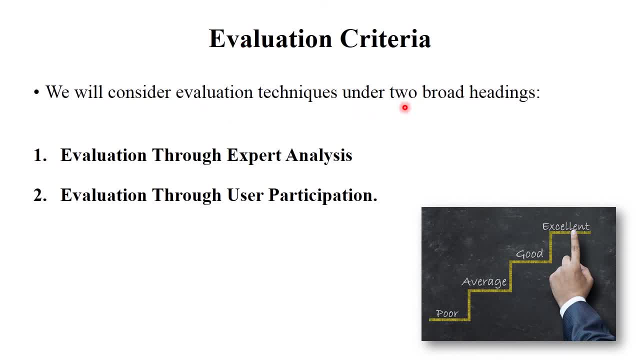 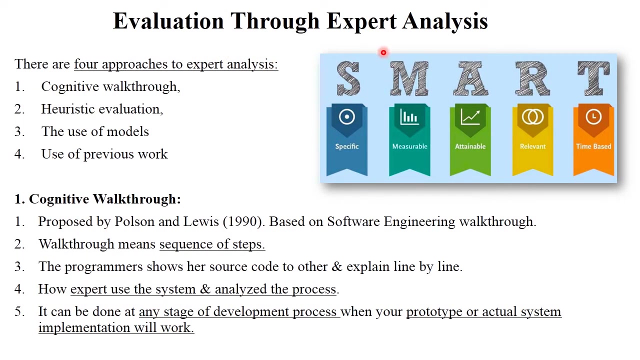 criteria. We will consider evaluation criteria under the two broad heading. The first criteria is evaluation through expert analysis and second, evaluation through user participation. okay, So evaluation done in both ways, through expert and through users Next. So next first is evaluation through expert analysis. There are four approaches in expert analysis. that is, cognitive work. 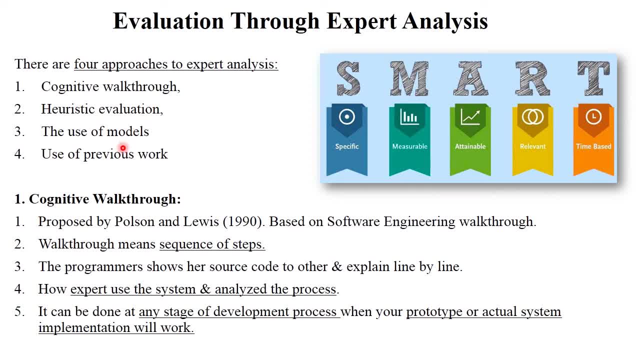 through heuristic evaluation, the use of models and use of previous work. There are four expert analysis, So let's see how exactly these work. The first analysis is through cognitive work, through Cognitive work through, proposed by Paulson and Lewis in 1990.. It is based on software engineering. 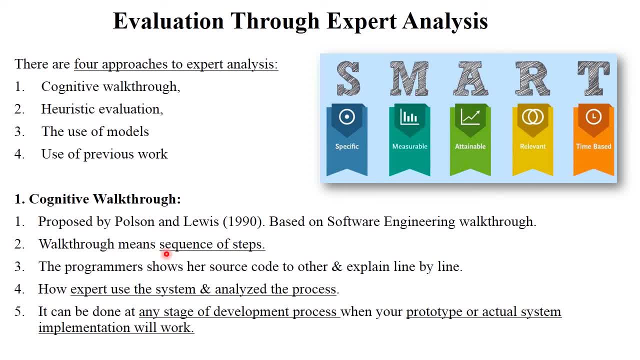 work through. What is mean by work through? Work through means sequence of steps In stepwise your algorithm or your will be worked. For example, the programmer shows her source code to other and explain line by line right. This concept is called as cognitive walkthrough. Means how expert use the particular 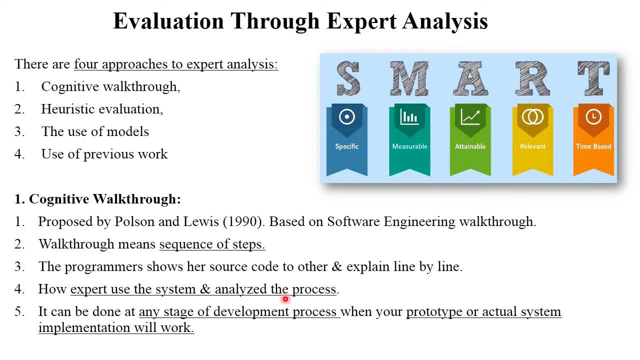 system and analyze the process. Each and every programming line there will be a comment is mentioned right. So comments are the most important way to analyze how exactly system will be worked and how exactly the particular model will be work. It can be done at any stage of development. 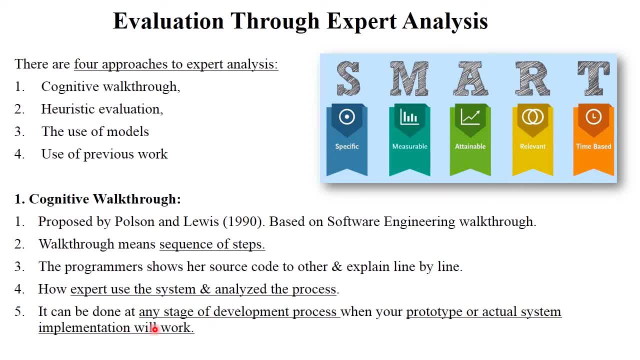 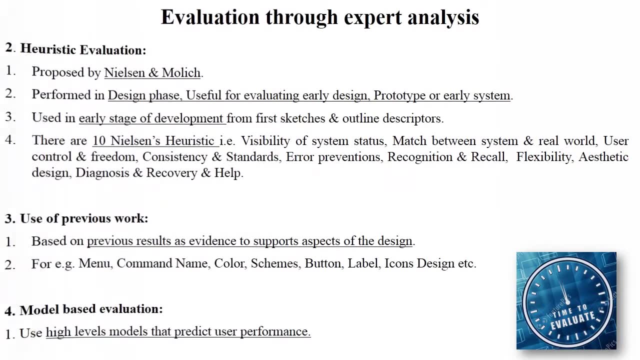 process when your prototype or actual system implementation will work. So this thing is called as cognitive walkthrough: Means to analyze or check the particular process through the expert in sequence. right, Okay next. The next is heuristic evaluation. Heuristic evaluation proposed by Nelson and Mollage. 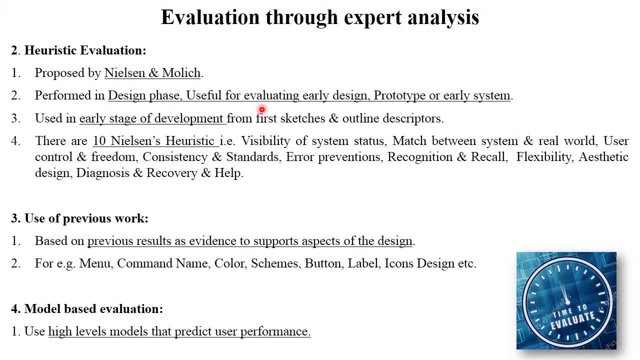 It perform only in design phase. It is useful for evaluating early design, prototype or early system. Heuristic evaluation used in early stage of development process. For example, I have explained Nelson's term heuristic in my last video. That is to check visibility of system, match your system. 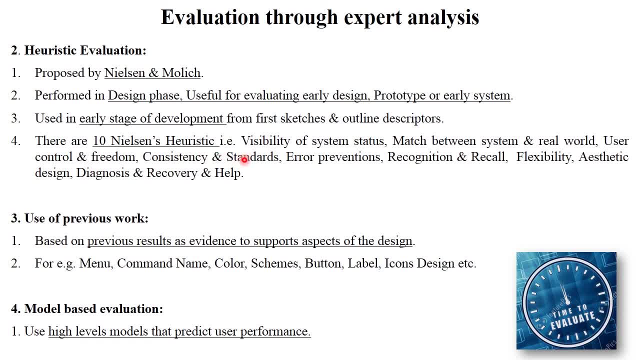 with real world, user control and freedom, consistency and standard of your design, error prevention, recognition, organization and recall, flexibility of your system, diagnosis, recovery and health- All those things I have explained in my last video. You should watch that. So these are the Nelson's term Heuristic, That Heuristic. 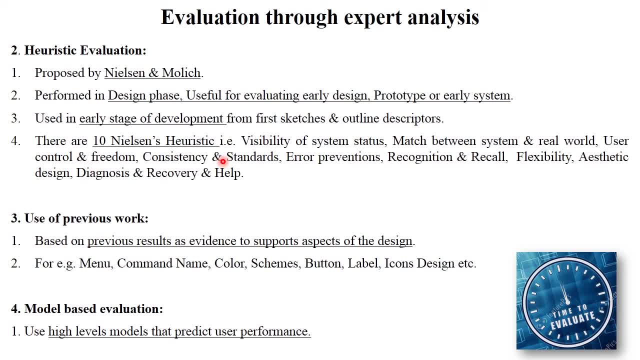 will be helpful for designing a particular product. So heuristic evaluation done in early stage, That is, suppose you design a particular software using paper pencil work, using sketch right, That is low fidelity, prototyping right. so this kind of concept is called as heuristic evaluation. if your design is good or 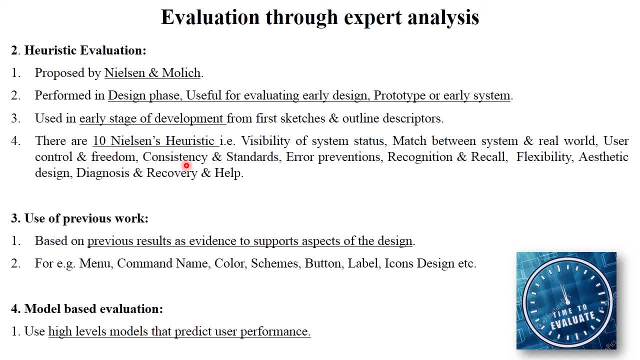 properly as per the requirement, then your implementation will be work. next, use of previous work. it is based on previous result as a evidence to supports aspects of the design. for example, if you press a particular button, so the first form will goes to next form. right, if you submit the? 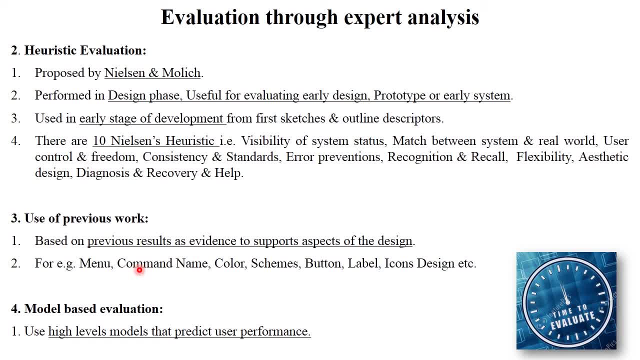 particular application that will be submitted and data stored into the database, right? so this is the concept of the use of previous work, means there is a particular sequence, right so? menu command, name, color scheme, button label, icons, design: you should analyze all those things. next, model based evaluation. 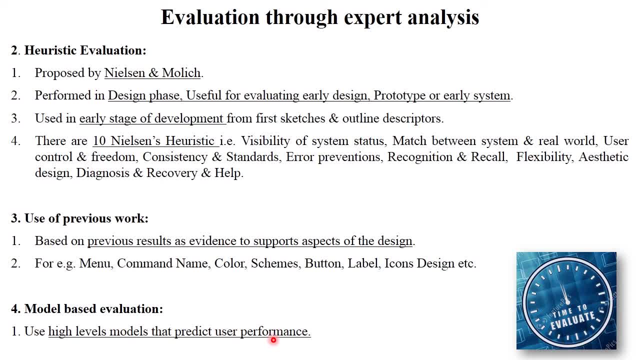 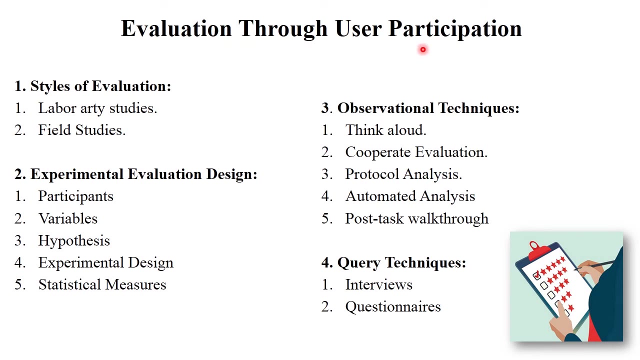 so use high level models that predict the user performance. always used latest framework, latest technology and high level model, which include different types of features in that. so this: all things are done by the expert. expert evaluate all those things clear. next, next evaluation through user participation: how user evaluate the. 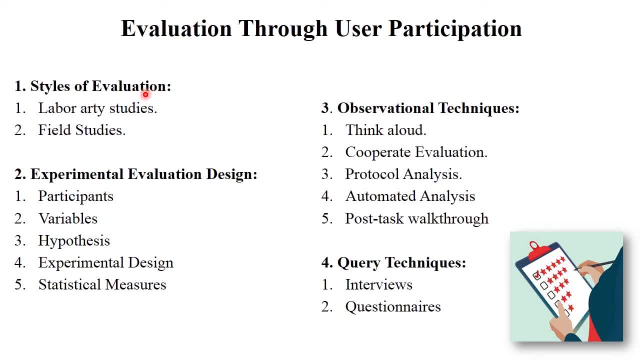 particular system. so styles of evaluation include laboratory studies and field studies. next, experimental evaluation design means user evaluate the participants. how much participant use the particular system? then variables hypothesis, experimental design and statistical measures. observational technique include think aloud. corporate evaluation. protocol analysis means there are some agreements or rules. you should check that particular agreements. then goes to: 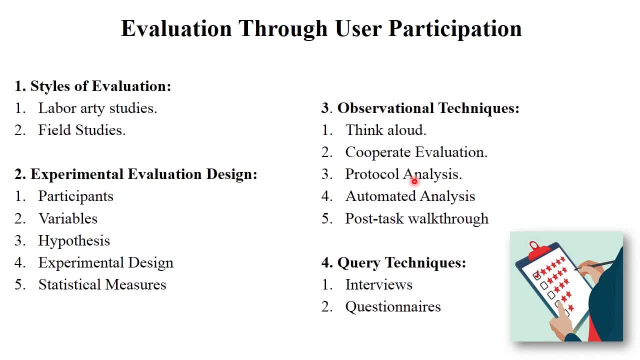 next page, right? so this system is called as protocol analysis, automated analysis and post task walkthrough. automated analysis means, suppose you sign up for string and after that you should log in by using ID and password. this thing is called as automated analysis, then cure technique, that is, interviews, questionnaires, etc. so these things or 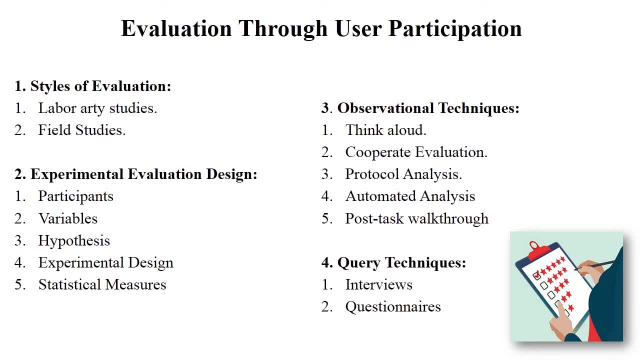 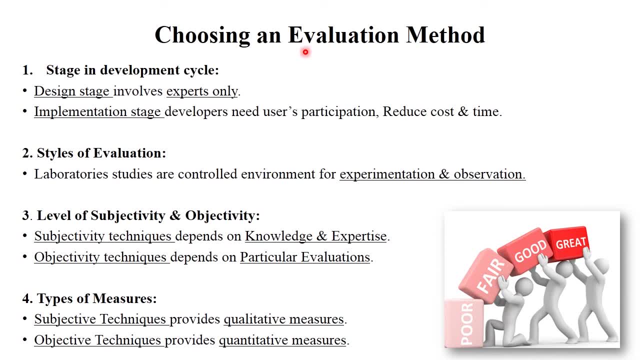 this evaluation are done by the user. next, the next, choosing an evaluation method. how exactly evaluation should done? the first stage in development cycle: in design stage it involves expert, only expert- analyst analyze the particular system design as per the user requirements. and in implementation stage, developer needs user participation right. that is, reduce cost and time. 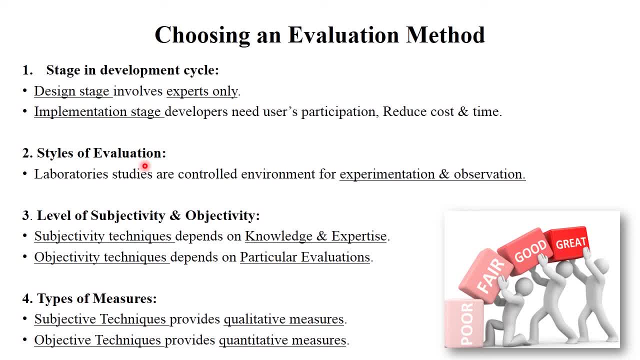 next, styles of evaluation. there are two styles of evaluation, that is, experimentation and observation. you should exactly develop a particular product and experiment it how exactly this will be work. and also observation: observe a particular system right. next level of subjectivity and objectivity. subjectivity technique depends on knowledge and expertise and objectivity technique depends on. 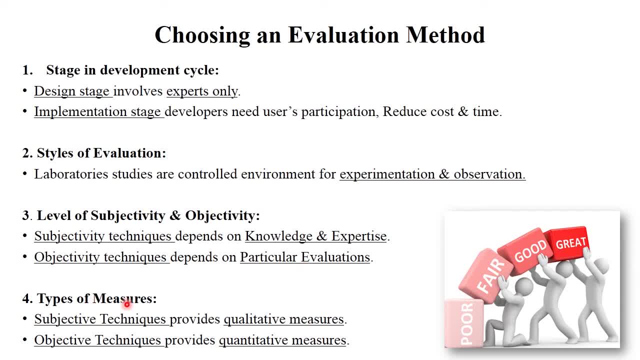 particular evaluation. right next, types of measures. subjective technique provides quality to measures, that is, exact quality of your product that will be measured. and objective technique provides quantitative measures. quantity means how many features you should involve in your particular product that will be matched with user requirements or not. right next next, information provided. there are two types of information, that is: 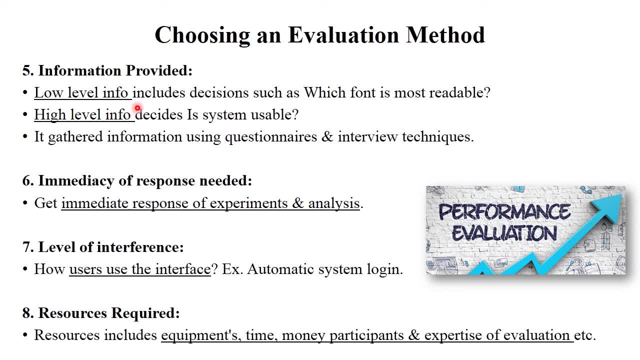 low level information and high level information. low level information includes decision, such as which font is most readable, which color is suitable right. and high level information decide each system. usable system is properly used is gathered. Gathered information using questionnaires and interview techniques. right, There will be a feedback system or rating system. right, 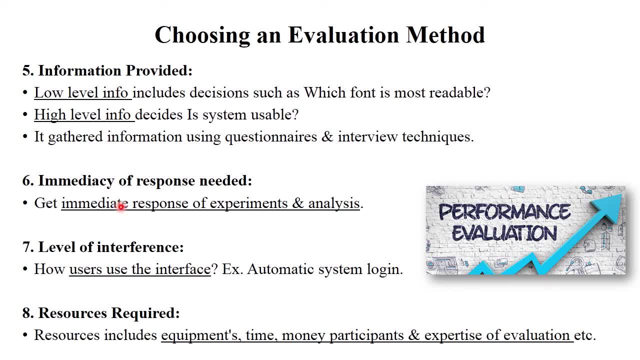 So this system is called as high-level information. Next, immediacy of response needed Means get immediate response of experiment and analysis. Then level of interference Means how user use the interface. For example, automatic system login, Automatic your Wi-Fi. 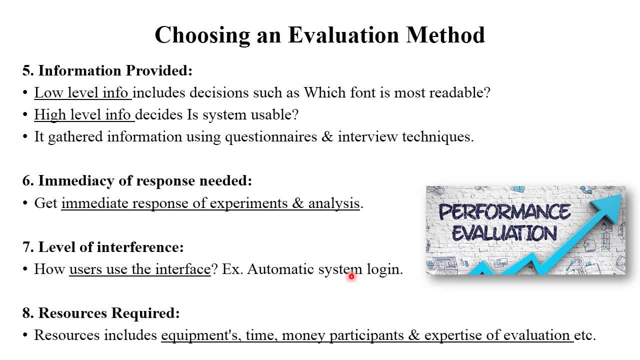 Suppose you should sign login a particular Wi-Fi, right? So next time you should check automatic login So it directly connected to your PC, right? So this system is called as level of interference. Then resources required.